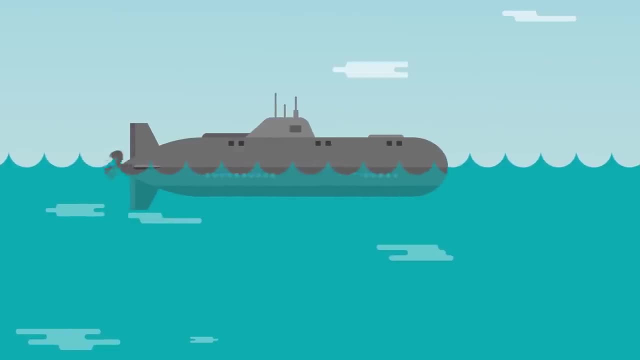 missile submarines to make up the United States Navy's arm of the nuclear triad Deployed in 1990 to replace the Trident C-4 missile. the Trident 2 has much greater range and accuracy than its predecessor. The cost of this greater range and accuracy is $3.6. 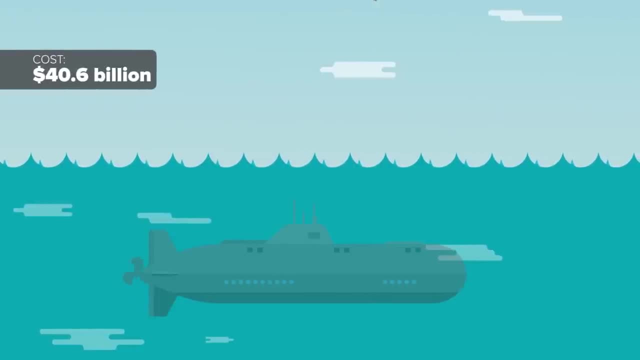 billion. This is one of the biggest challenges US nuclear equipment faces to the American military. The UGM-133 Trident II is a more effective missile program than the UGM-133 Trident. accuracy is $40.6 billion. The missile is able to travel at approximately 18,000 miles per hour, or 24 times the speed. 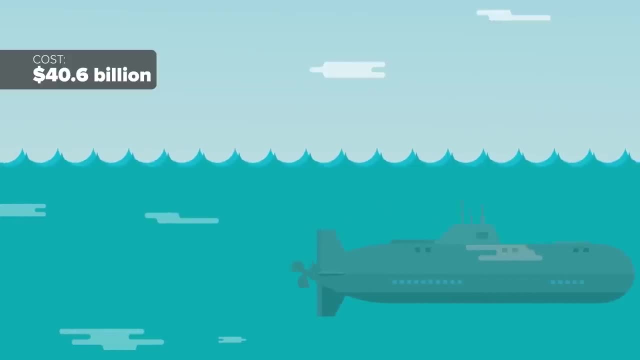 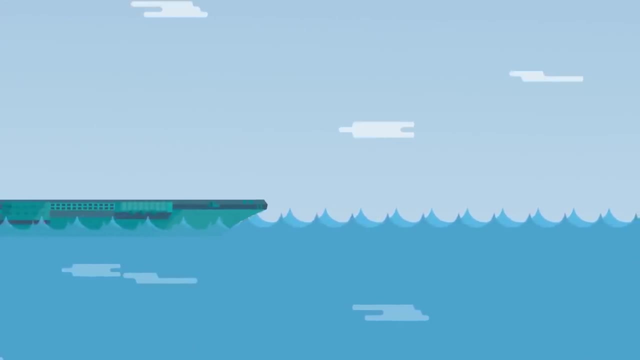 of sound and carry a nuclear payload of up to 14 thermonuclear warheads per missile. 8. The CVN-78 aircraft carrier, or the Ford-class carrier, after the lead ship of the class, is currently in production to replace the Nimitz-class aircraft carrier. 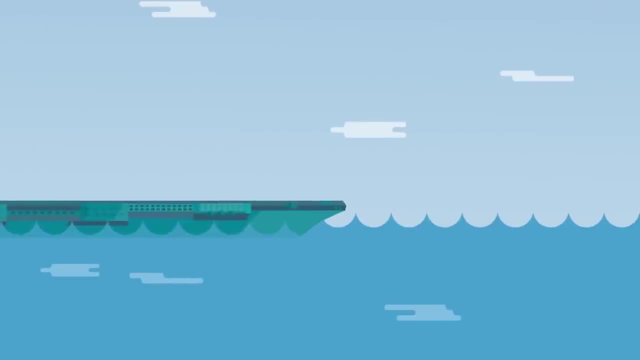 So far the lead ship, USS Gerald R Ford, and the USS Theodore Roosevelt, have launched in a program expected to cost $42.5 billion. The Navy would argue it is getting a bang for its buck in its replacement of the Nimitz-class. 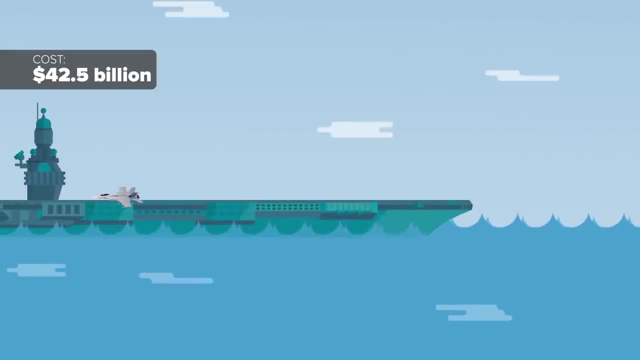 which launched in 1970.. The Ford-class can carry up to 90 aircraft and sail for 90 days without being resupplied. Each ship in the class is expected to have a service life of 50 years and act as a key part in power projection for the United States military around the world. 7. The F-A-18 Super Hornet carrier-based multirole fighter was the United States Navy's replacement for the F-14 Tomcat, now serving alongside its brother, the F-A-18 Hornet, in serving on today's Nimitz and Ford-class aircraft. 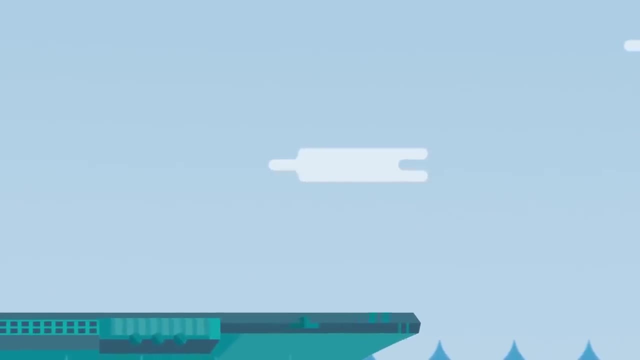 The total program costs reached $51 billion, costing twice as much per aircraft as the F-A-18 Hornet. For the doubling of cost, the Navy did get several upgrades. The airframe is slightly larger but also uses fewer parts, increasing the simplicity. 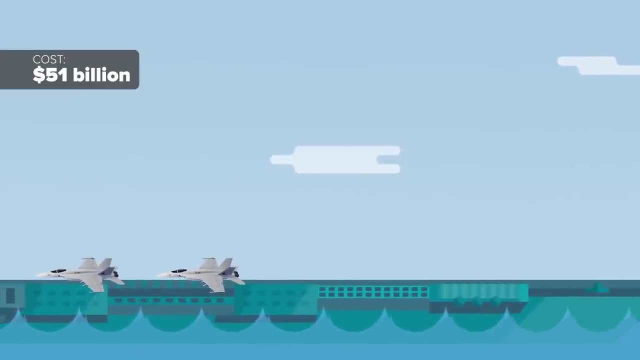 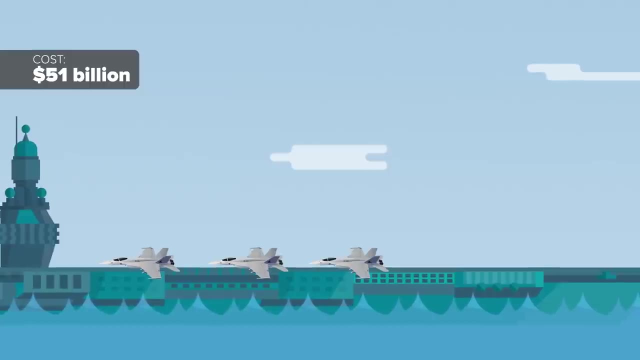 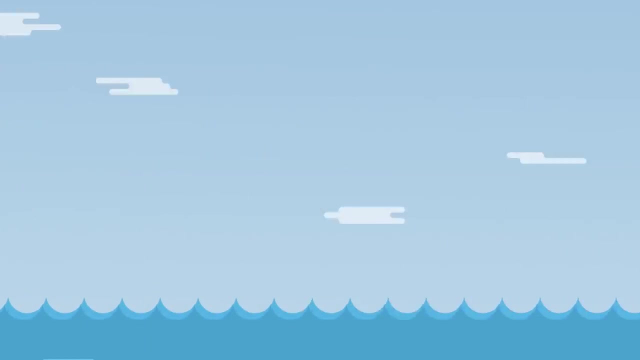 of the design while improving the aerodynamic effectiveness of the place. The internal fuel capacity was also increased by 33%, which expanded mission range by 41%, and the Super Hornet receives a suite of new and improved electronic systems. 6. The Boeing KC-46 Pegasus is an air refueling tanker and transport aircraft for the United. States Air Force, Based off Boeing's 767 airliner. the first of the new aircraft was expected to be deployed in 2016,, with the first full batch of 18 combat-ready planes expected to be delivered by early 2018.. The KC-46 is being used to replace the quickly aging KC-135 Stratotanker. 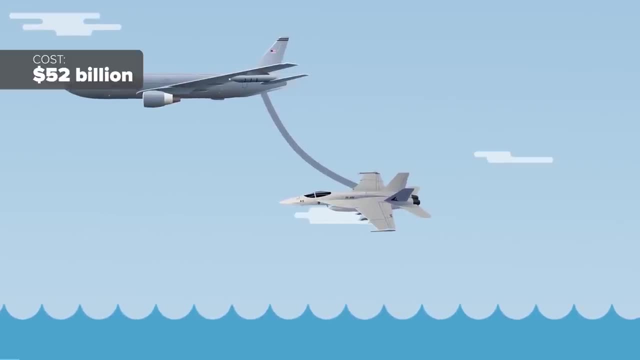 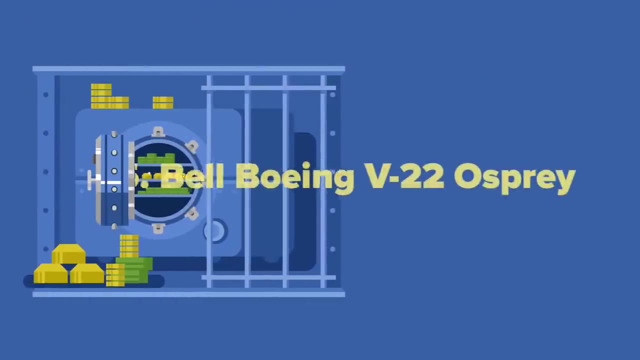 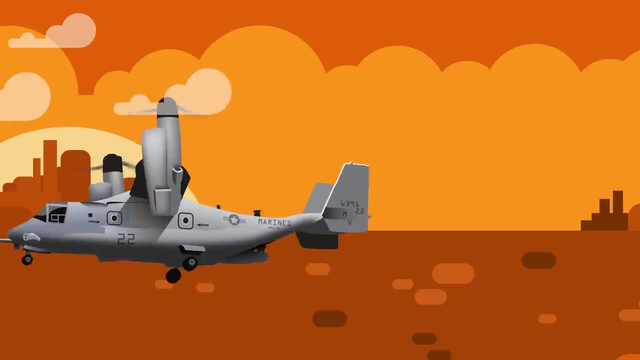 The program cost has entered $52 billion, but does have notable advantages in both cargo and aeromedical evacuation capabilities. 7. The Bell Boeing V-22 Osprey has its origins in the failure of Operation Eagle Claw during the Iran hostage crisis of 1980, where the United States Armed Forces decided it needed. 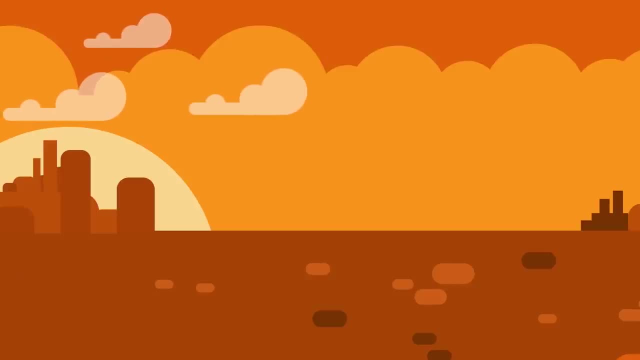 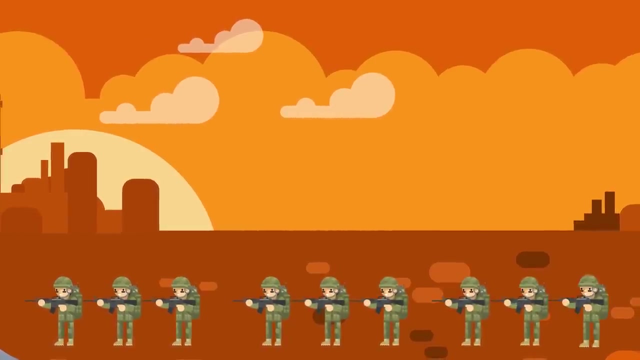 an aircraft that could carry troops long distances quickly while having the functionality of a helicopter. Fast forward 27 years to 2007,, when the V-22 Osprey was officially deployed by the United States Marine Corps, followed by the US Air Force. 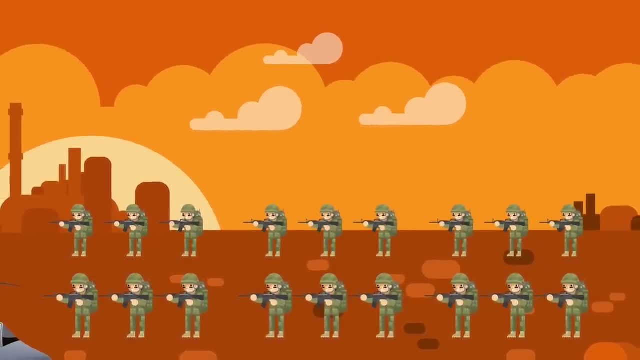 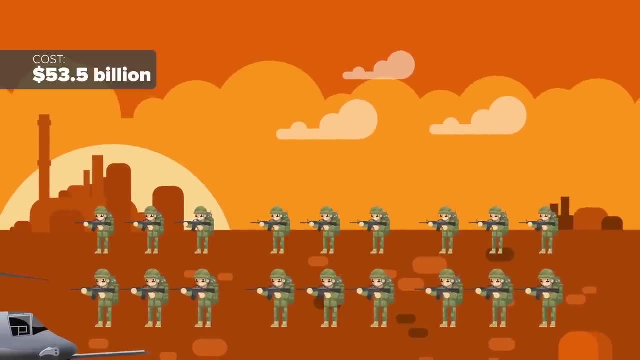 The program was, for a long time, the poster child of cost overruns. The program was designed to be a multirole destroyer with a capacity of up to 3.5 tons and efficiency, eventually costing $53.5 billion. This despite being repeatedly noted that the regular helicopters could be had with the 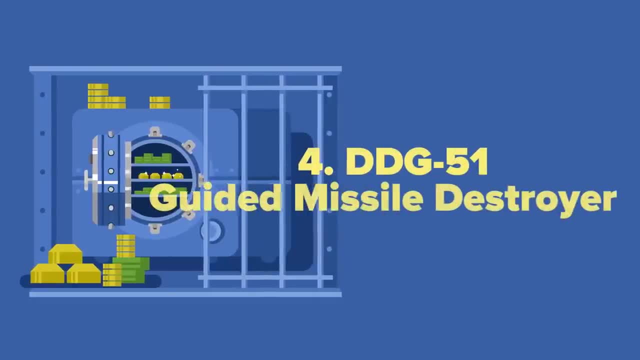 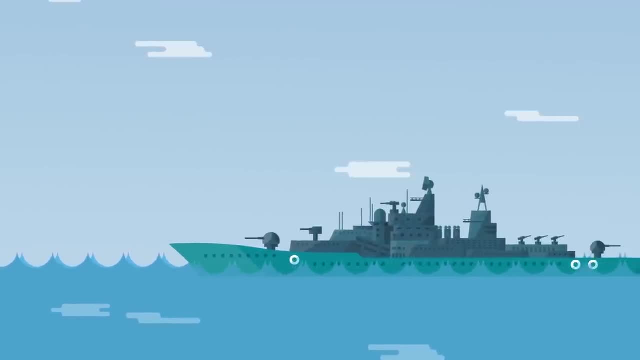 same capabilities for half the cost. 4. In production since the 1980s. the DDG-51 Arleigh Burke-class guided missile destroyer was developed as a multirole destroyer to utilize many new combat systems developed shortly before, including the Aegis defense system and the Tomahawk cruise missile. 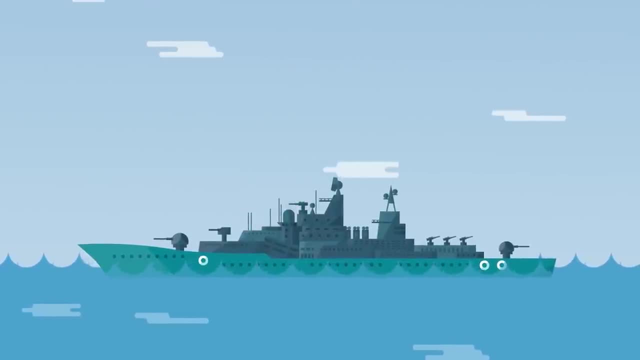 After the first ship of the class was officially commissioned in 1991, it has become the only destroyer in the United States Navy, Despite being in service 26 years. the Navy is planning on purchasing a third group of the Arleigh Burke-class. running program costs up to $87.3 billion, with more spending in 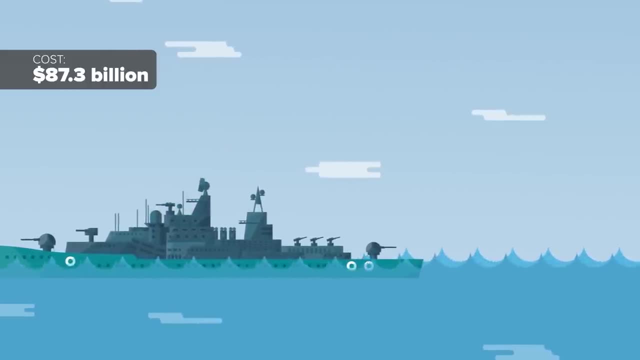 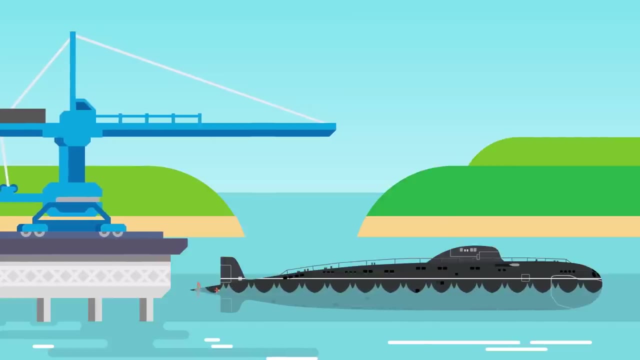 the future. That makes the Arleigh Burke destroyer one of the most expensive and longest running programs in United States military history. 3. The Columbia-class of ballistic missile submarine is in development as the replacement home to the United States Navy submarine-based nuclear missiles from the current Ohio-class. 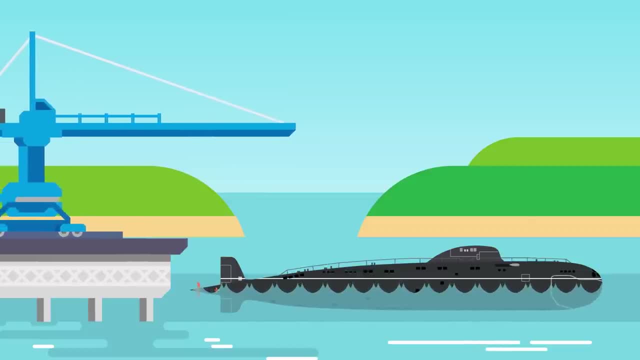 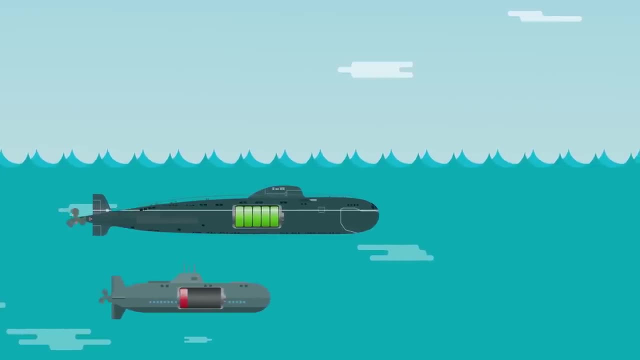 submarine 4.. The Columbia-class submarine is expected to launch in 2031, exactly 50 years after the first of the Ohio-class submarines launched. The Columbia-class will have 16 missile tubes and will never need to be refueled during. 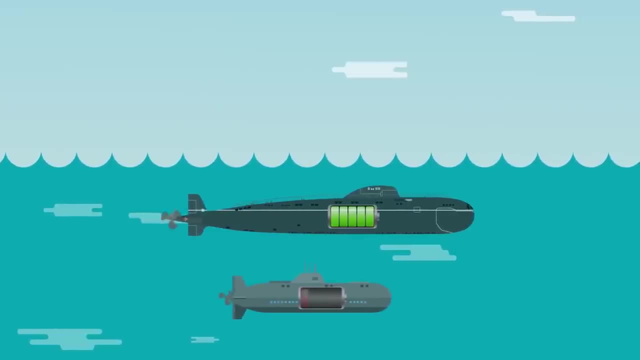 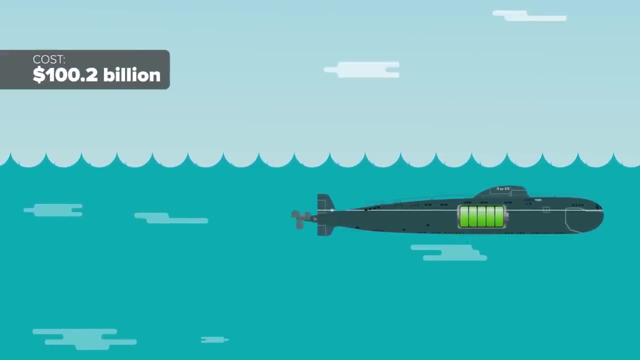 its expected 42-year service life. The Government Accountability Office released a report expecting the total acquisition cost of the class to be $100.2 billion and expect it would be another over $100 million per year per submarine in maintenance 2.. 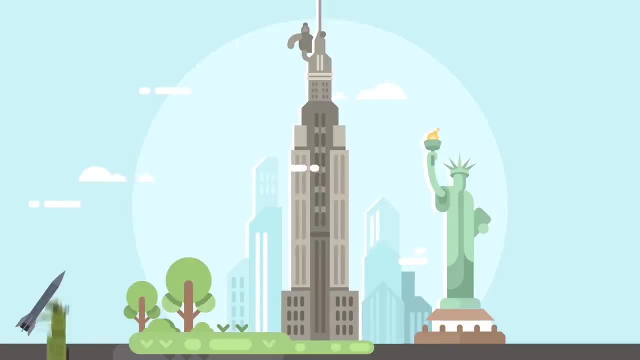 3. The Columbia-class missile defense system is a sprawling program geared towards stopping incoming missiles, including detection all of the way through interceptors. This program includes the Patriot missile defense system currently deployed in Israel, and the Terminal High Altitude Area Defense System, better known as THAAD, that is currently being deployed to South Korea. Although it originated in President Ronald Reagan's Star Wars, the program is still technically in the development stage and may one day include space-based and laser defense systems. So far, the program has cost $126.2 billion, and it is currently unknown just how much.